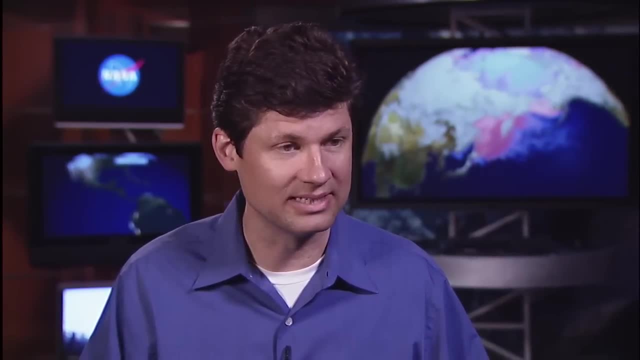 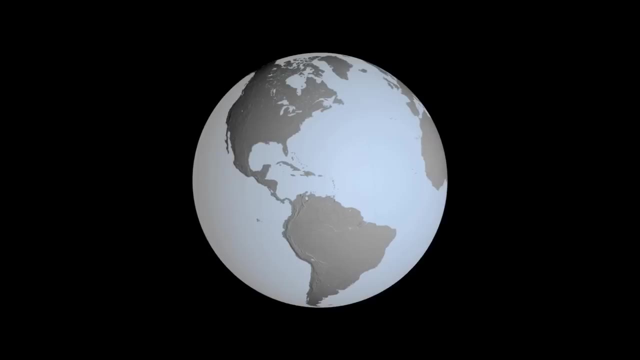 of that ice is also important, And in 2009, what we also released were some new satellite results where, for the first time, we were able to figure out what the thickness of the Arctic ice is all over the place, And what we're finding is that it's thinner now And that 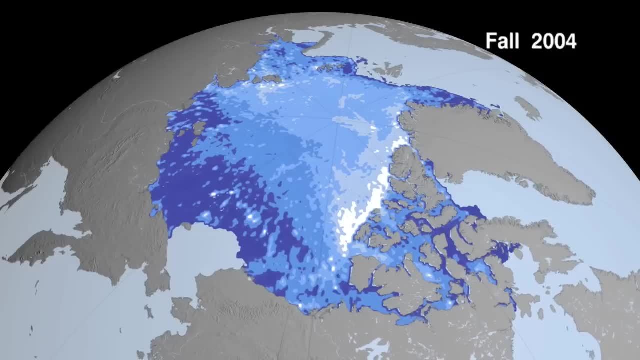 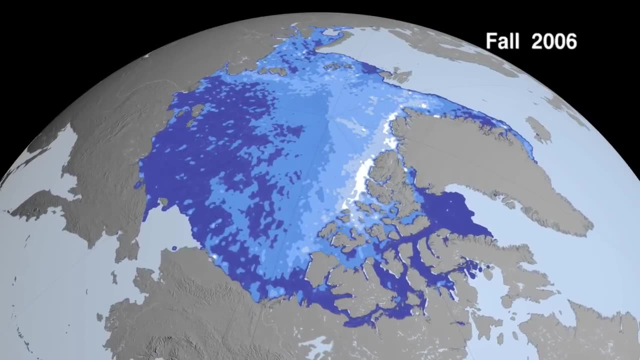 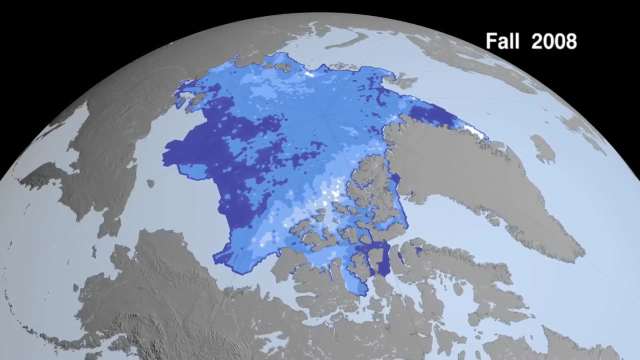 also, thinner ice is easier to melt than thick ice, And so all of this is setting the stage for predictions of an Arctic that is ice free in summer months somewhere in the coming decades. Now, we don't know when it's going to happen, but it's the kind of thing that a lot of people 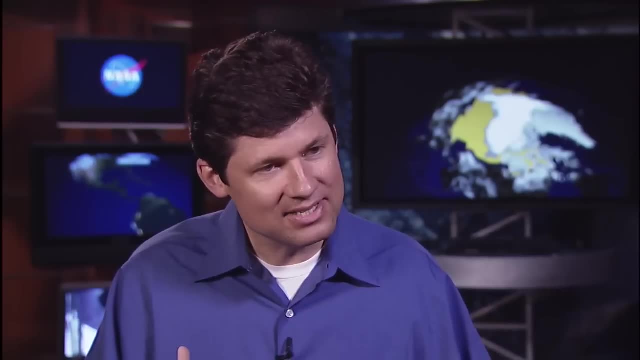 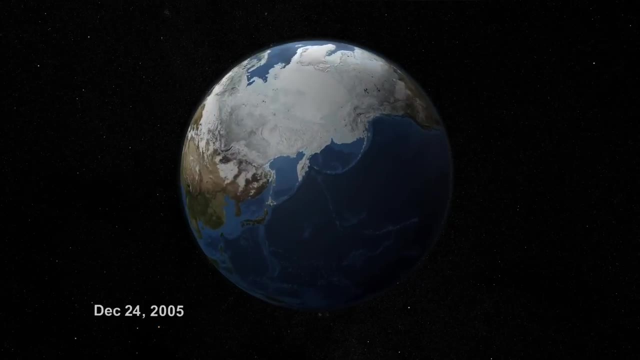 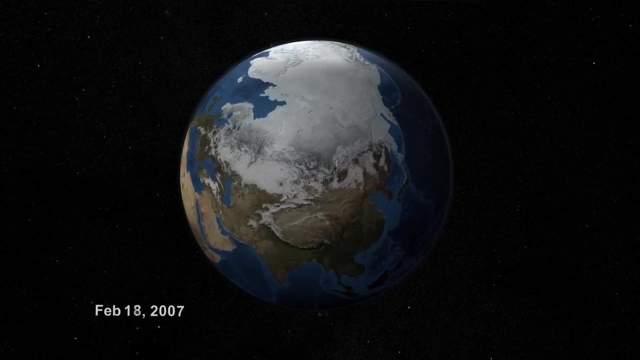 are working on trying to model, But it's so obvious that this is happening that people that live in the Arctic regions and the countries that border the Arctic are planning facilities based on their beings. There are people building warm water ports. There are oil companies preparing to do exploration. 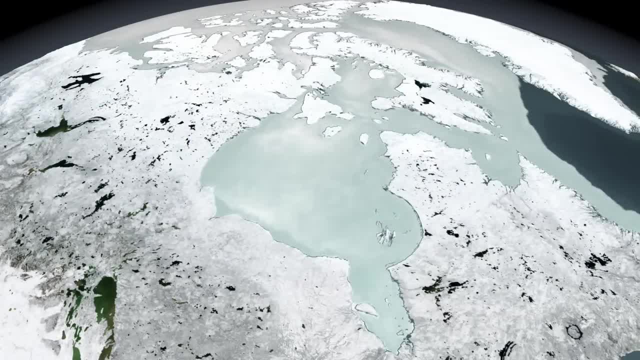 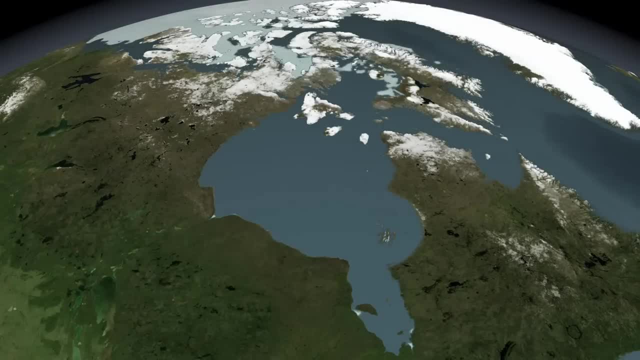 People talking about using it as a transportation route, But also the Arctic peoples that live there. they're observing these changes And they're saying things like: hey, we used to be able to walk out on the sea ice and now we can't do that anymore. So these changes? 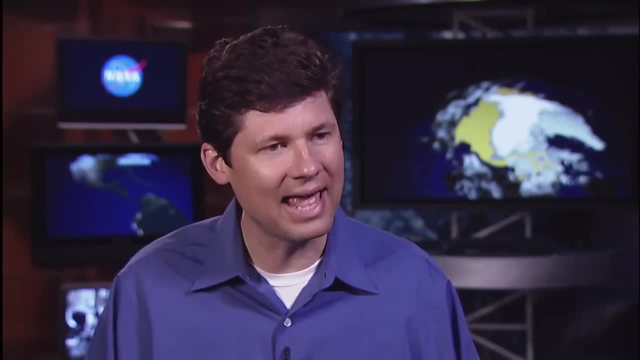 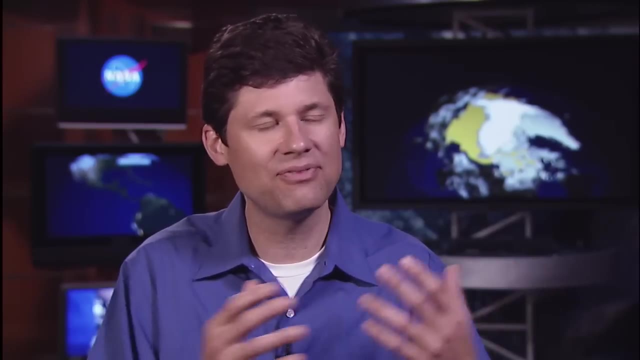 are real and they're happening, And what we're trying to do at NASA is, like I say, to go out and characterize this ice, understand how it works. How is it affected by ocean currents, How is it affected by wind? How is it affected by winds, How is it affected by sunlight, So that we can correlate that. 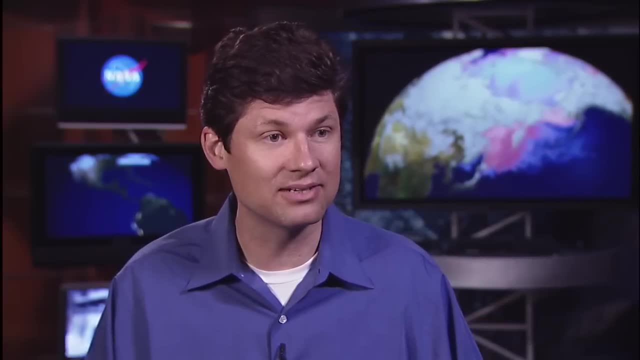 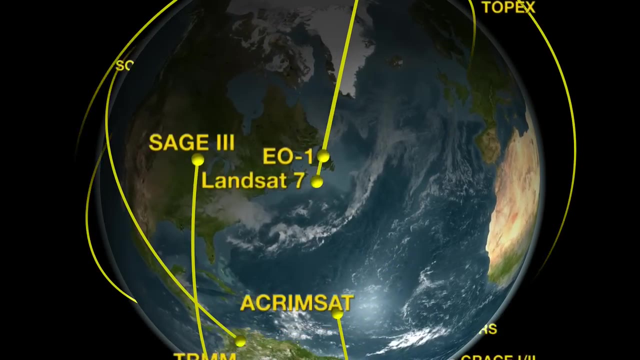 with the changes we see in the atmosphere and develop better predictive models. We study the Arctic sea ice with a range of tools. The most important tools are satellite tools. You need to think of this ice as being continent scale. okay, This isn't something. 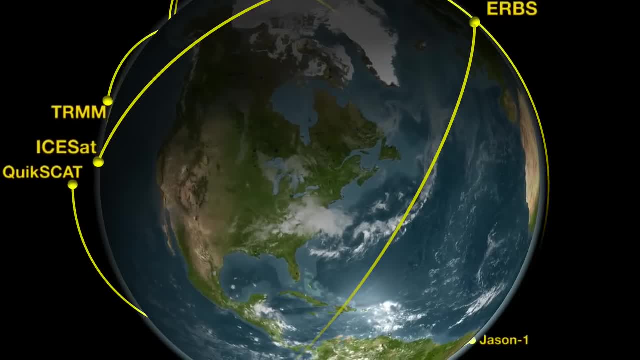 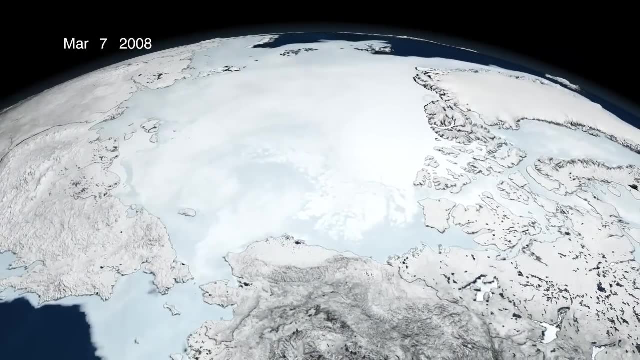 that you can get with a single aircraft flight. And that's why NASA is really important, because we operate the satellites you can study it with, Because from that we can tell what the concentration of ice is. You know, is it ice that's a foot thick, that's covering everything, or is it little patches? 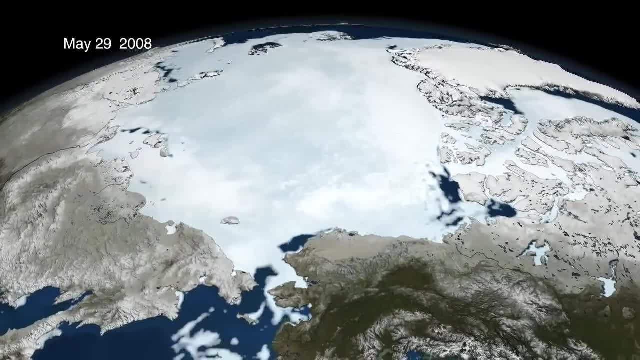 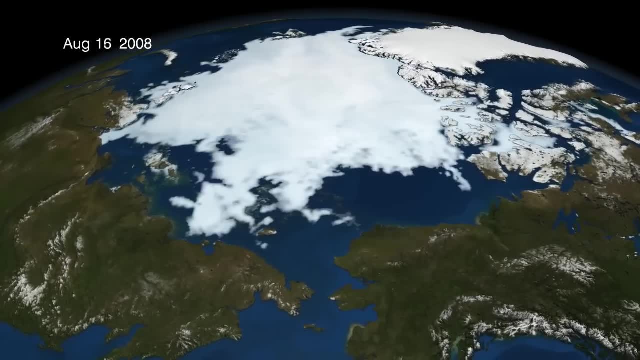 of ice. But that's not the whole story. We also need detailed studies. We're interested in how rough is the surface This ice is. in some places it's smooth, like that pond in the Midwest that freezes every winter, But in other cases that ice has been blown and crunched.